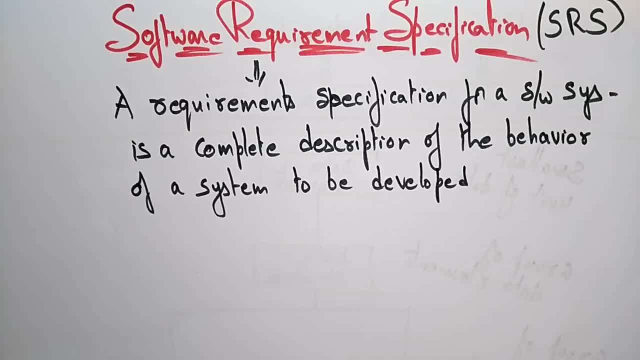 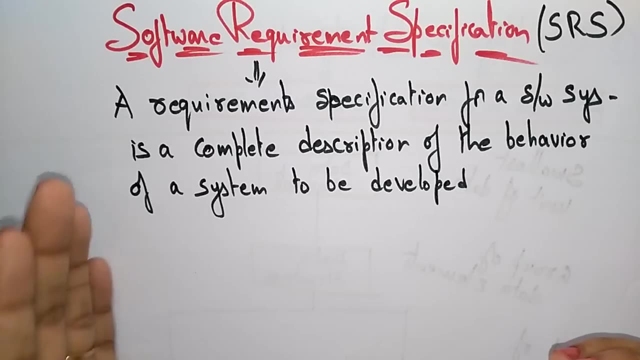 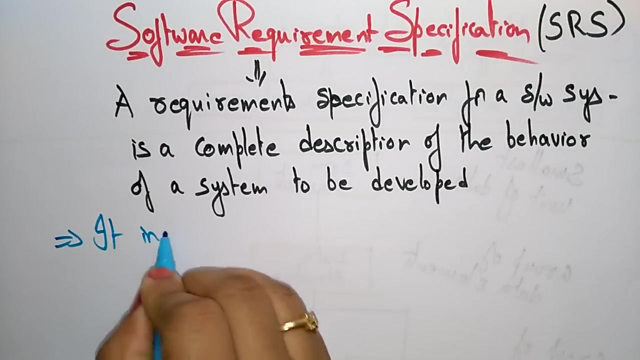 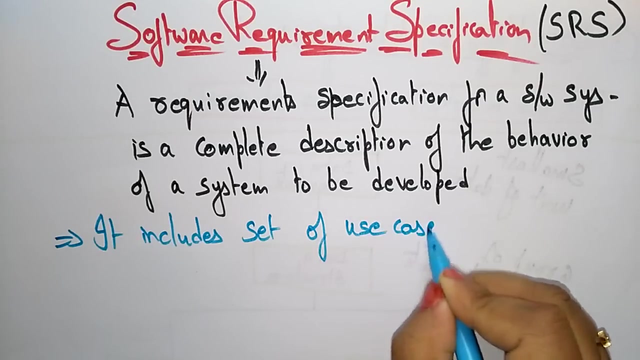 Means it gives the description about the system that is going to be developed, So that complete information, complete description, the description will be stored in the form of, will be implemented in the form of SRS documentation, Software requirement specification. So this software requirement specification includes it includes set of use cases. 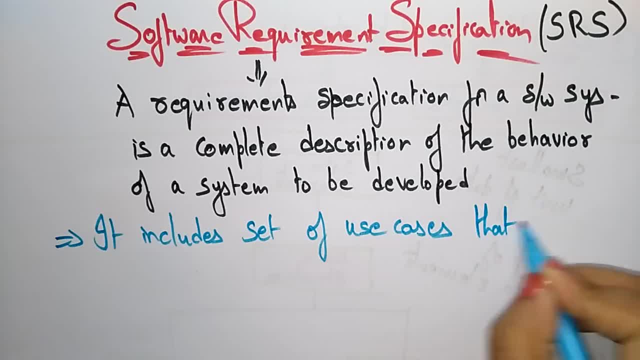 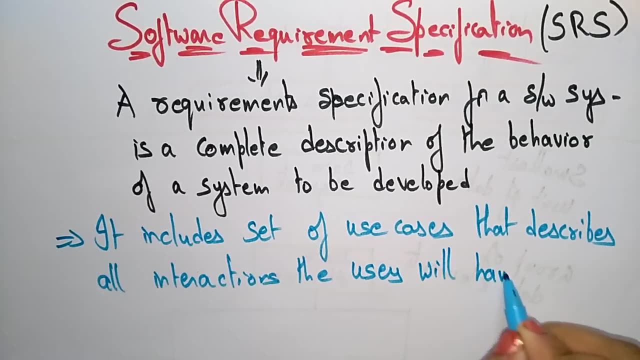 It includes a set of use cases that describe. that describes all, all interactions the uses will have, transactions the uses will have with the software. so this software specification requirement includes a set of use cases, What this uses cases will do. it describes all the interactions the uses will have with the system. 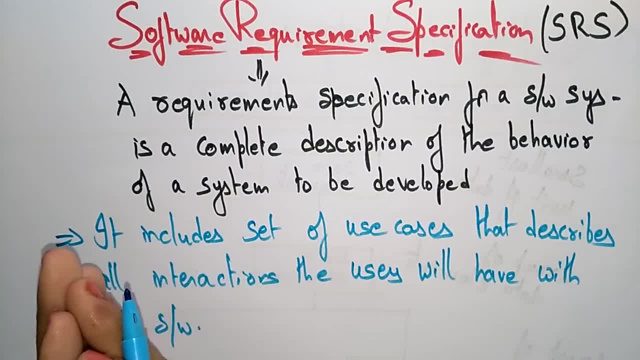 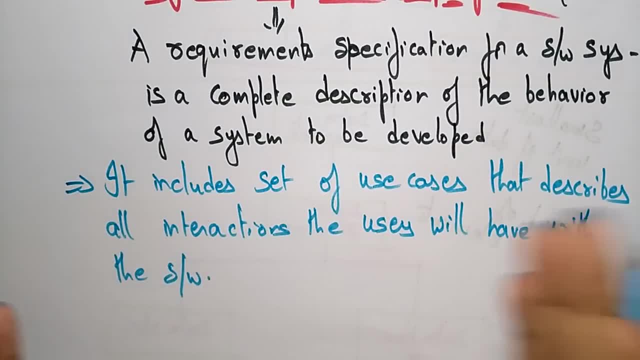 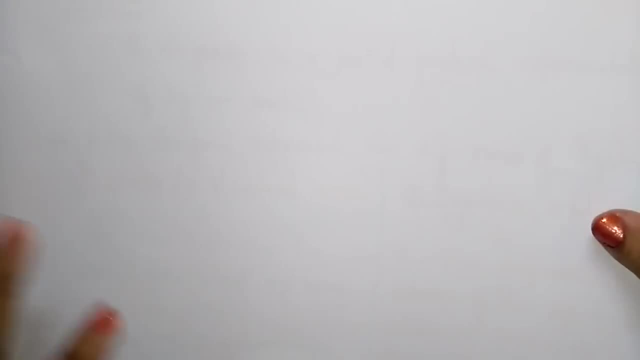 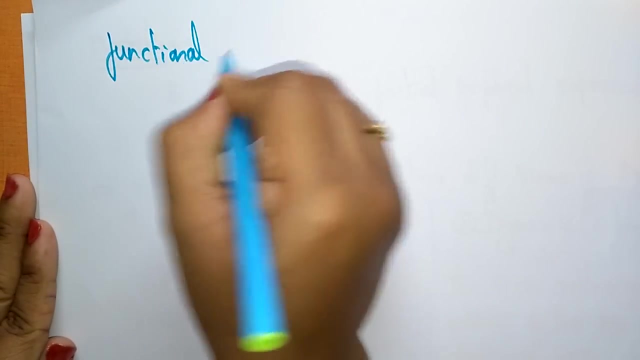 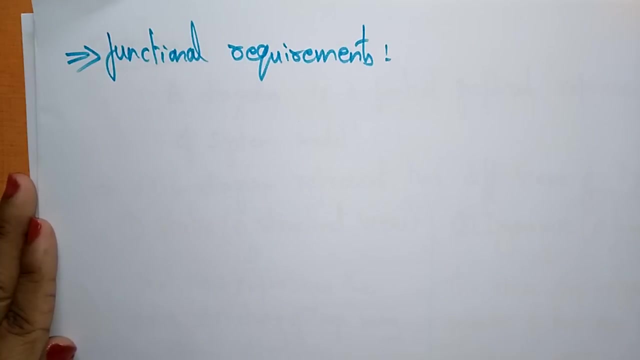 So these requirements reflect the needs of customers for a system that helps to solve some problems. The software requirement specifications may be consisting of functional requirements and the non-functional requirements. Let me explain that The software requirement specification consists of functional requirements. So what are those functional? what do you call this functional requirements? 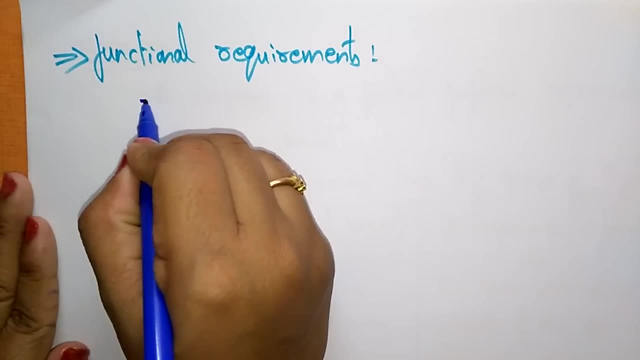 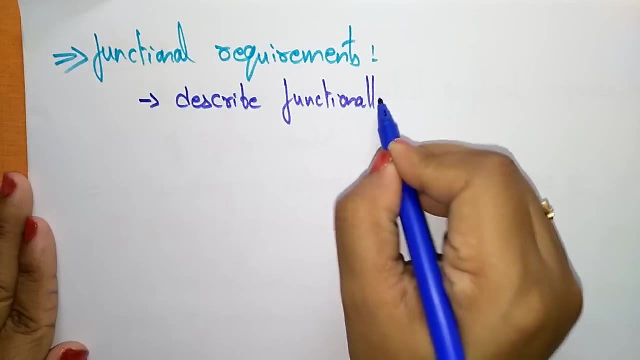 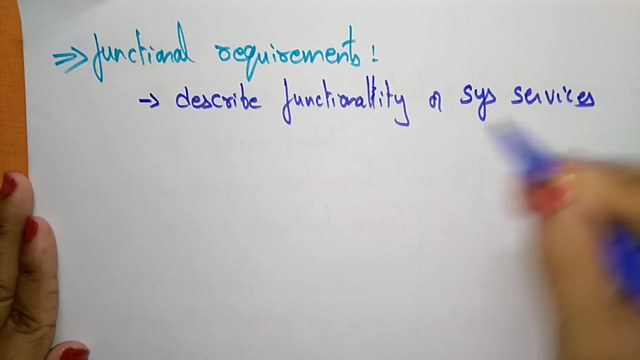 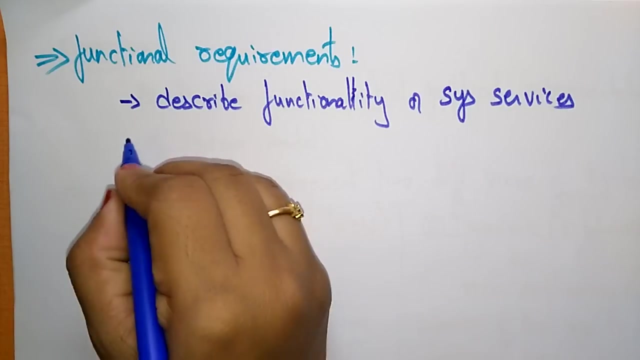 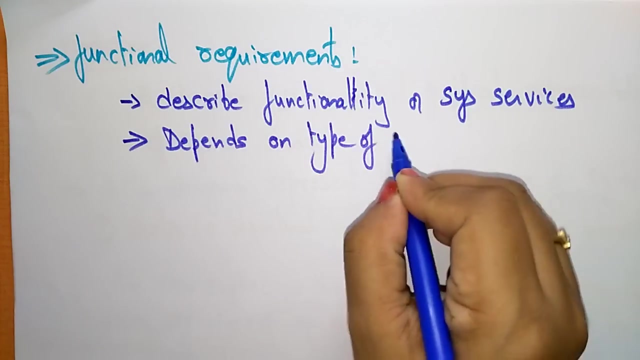 Functional requirements means it describe functionality or system services. The functional requirement describes the functionality of a system or a system services, And it depends on type of software and expected uses- Type of software we are using and expected uses. And what about the non-functional requirements? 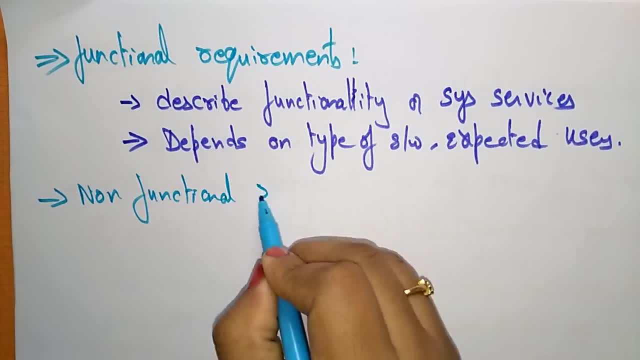 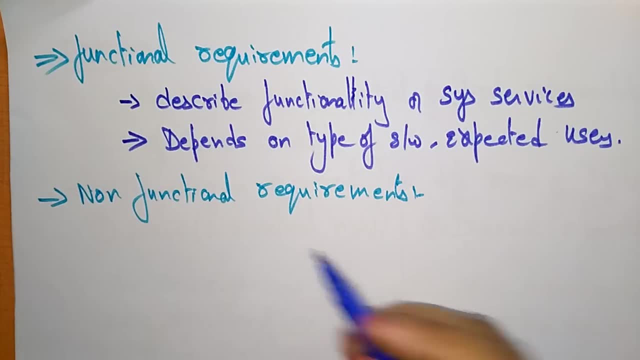 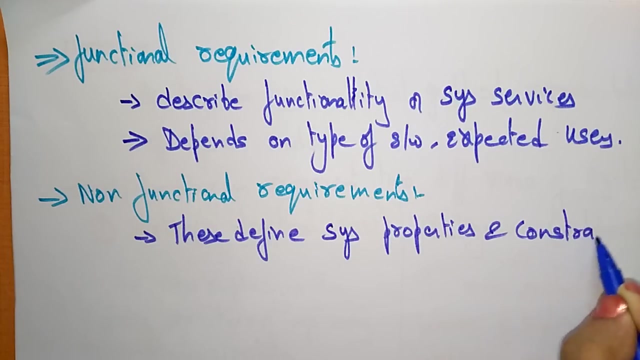 What are the non-functional requirements that are used in the SRS documents? What terms that will come under the non-functional requirements? So these defines the These. These define system properties. it explains the system properties and constraints. So functional requirements deals with the system services and whereas a non-functional 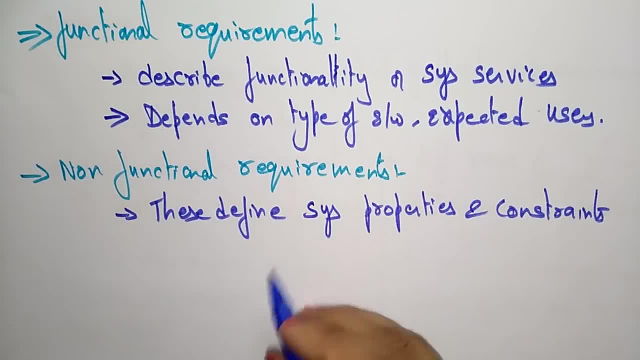 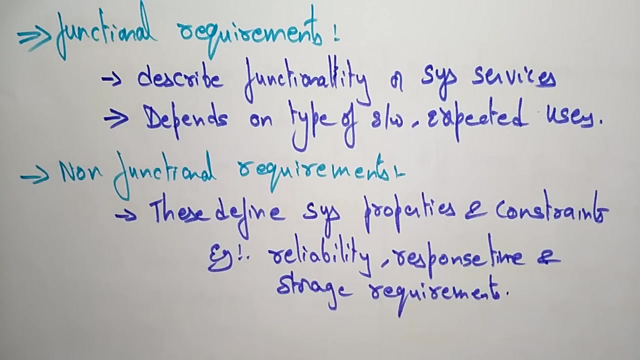 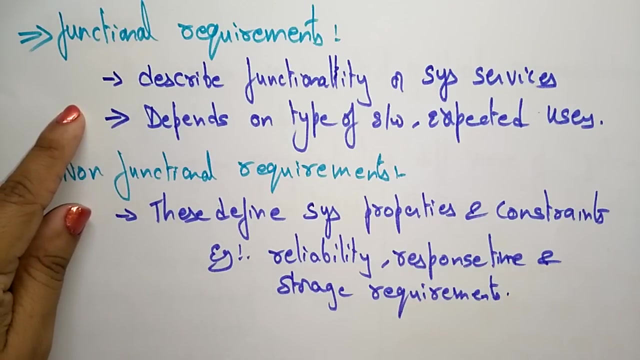 requirement defines the system properties and constraints. So the examples for these system properties and the constraints is reliability of a system, reliability, response time And and storage requirements. And one thing we have to be remembered: that it may be more critical. it may be more critical means a chance of this. non-functional requirements is more critical than compared to the functional requirements. 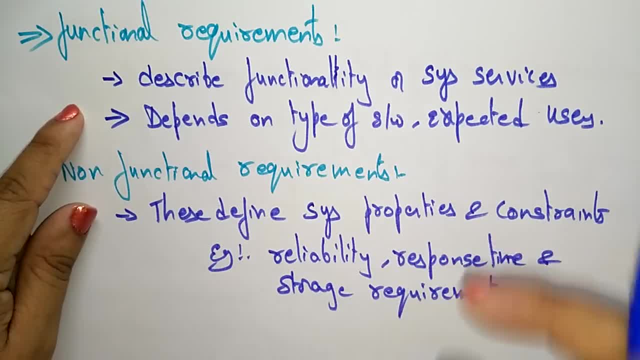 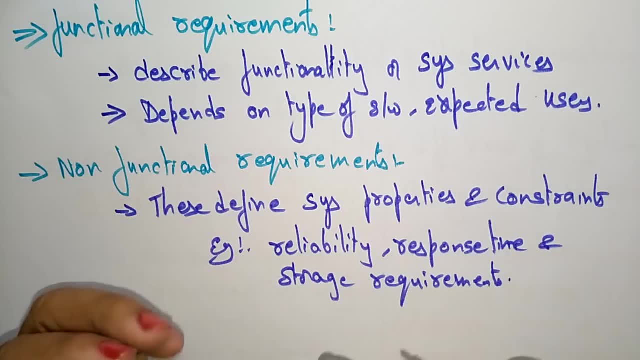 if there are non-functional requirements are not not up to the point, System is useless. Because if you didn't actualy realizbilty condition of the system, have the good response time and if you don't have the storage requirement, then your system is. 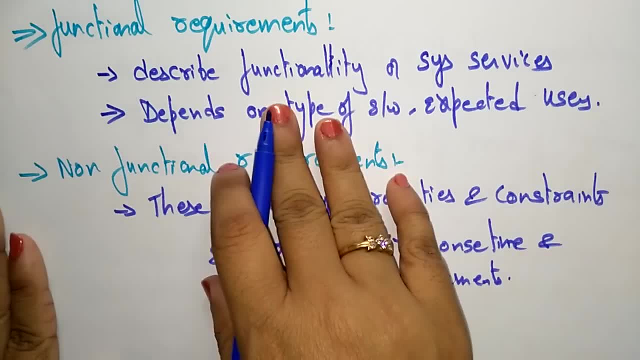 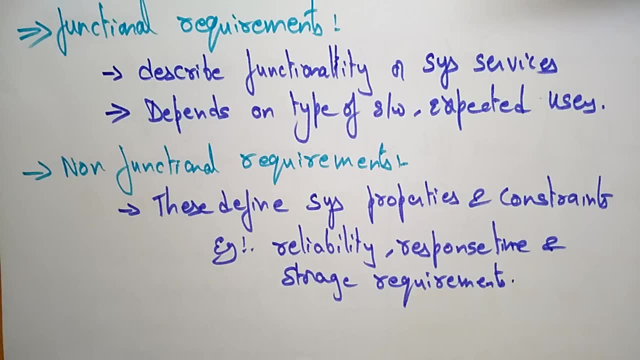 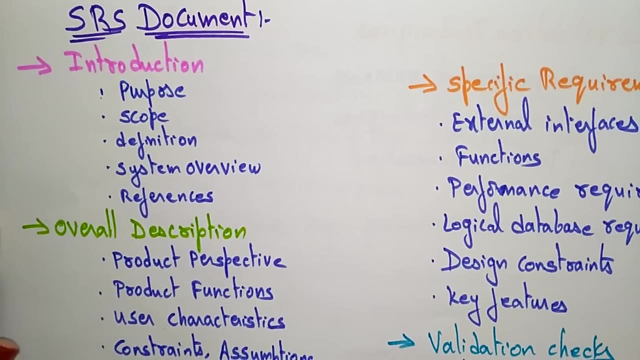 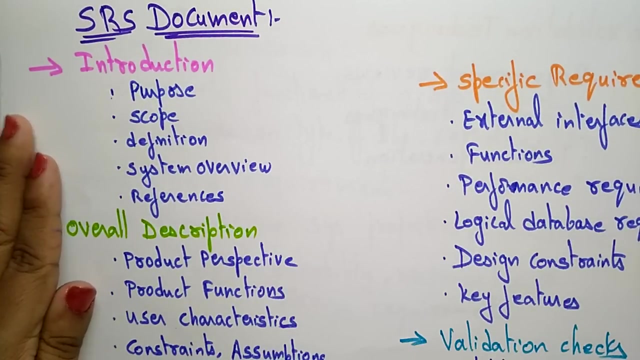 somewhat, it is useless. so, when compared to the functional requirement and non-functional requirements are more critical. okay, now let us see, uh, what the exactly the srs document consisting of the software requirement specification document consists of. so the first step, uh, in the documentation you have to write the introduction. in the introduction you have, you need to cover. 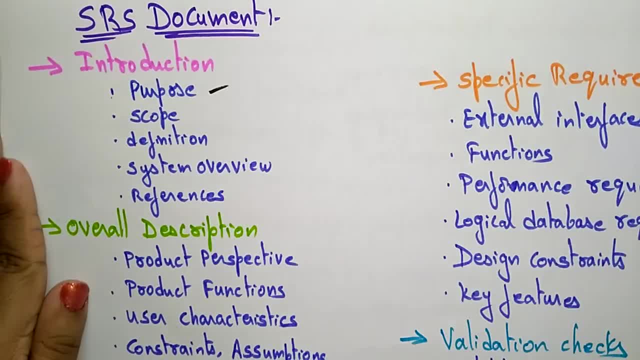 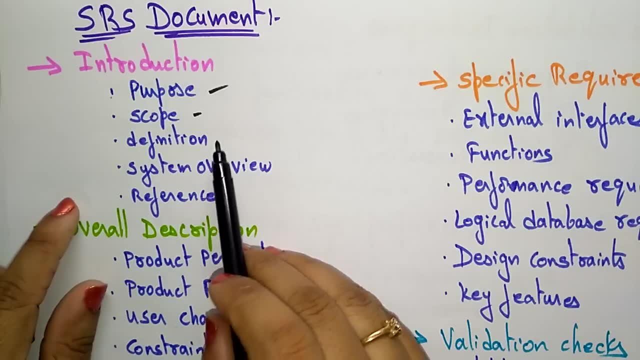 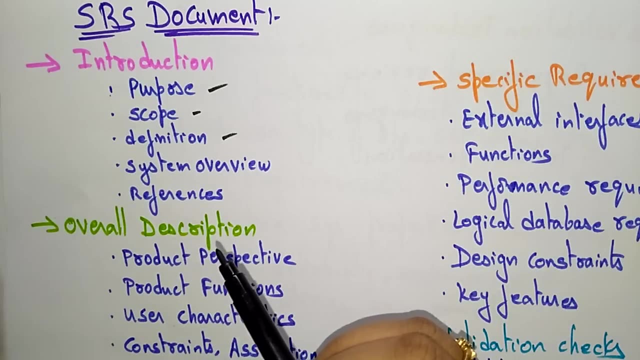 the purpose of your project, what is the purpose of the project and what is the scope of your the project? so, when you're going to be complete, and the definitions, uh, what are the synonyms, acronyms, that will be included in the definitions? the names that are, uh, the new names that are present? 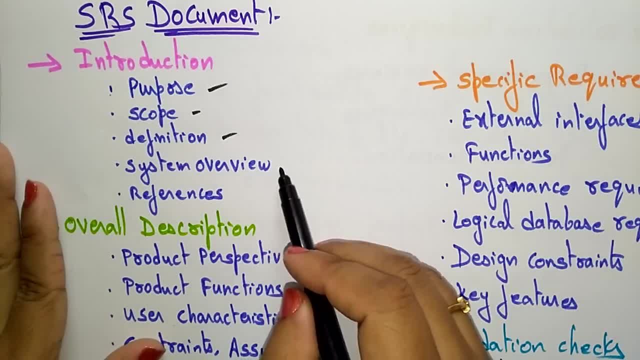 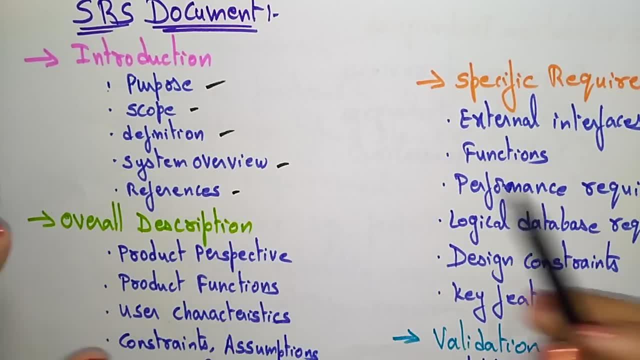 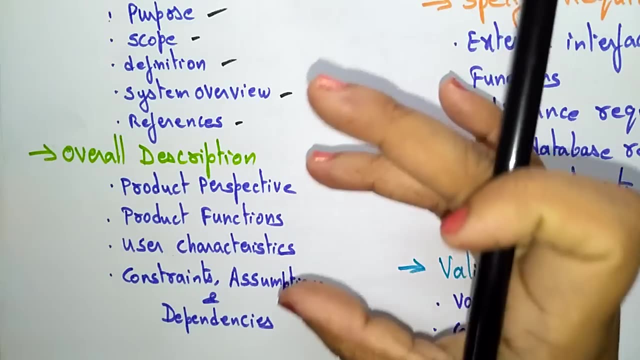 in the document uh project system overview. so the everything the system overview will be covered in this introduction part, and the references that you are using- so these are all- comes under the introduction. okay, once i have completed the introduction, now shift to the overall description of the system. in the overall description of the system you need to cover the product perspectives. 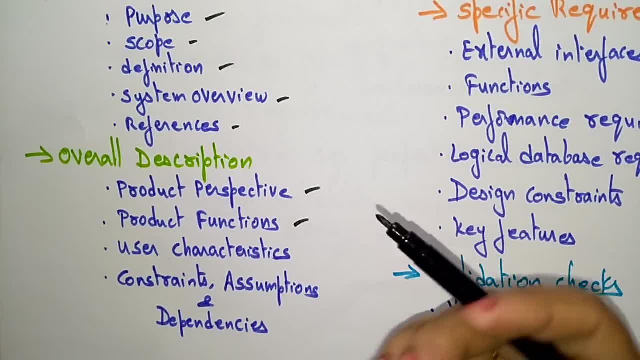 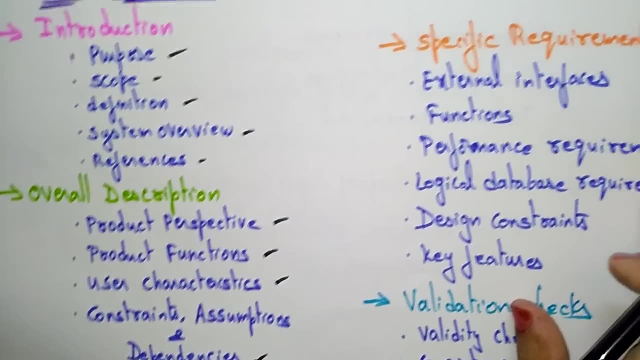 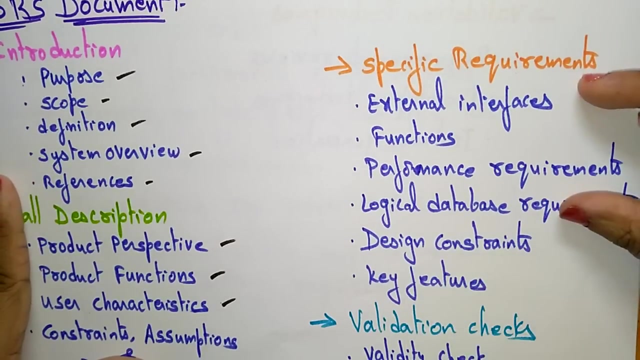 product functions. so the product that you are going to be developed, that product perspectives, product functions, user characteristics- what are the user characteristics in the system? constraints, assumptions and dependencies. everything will be covered under the overall description. so, after completing the overall description, try to write the specific requirements that you need to develop a product, the specific requirements that you need to